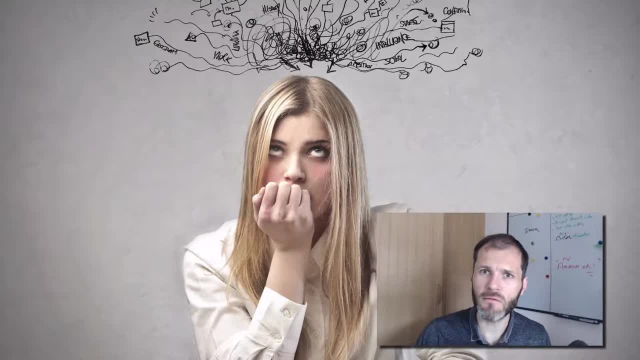 years ago, or 10 years ago, or even longer than that, and reflect on it, and reflect on what this event meant to you then versus what it means to you now. It could be something life-changing, like the time you got married or divorced, or it could be something smaller, like the time you. 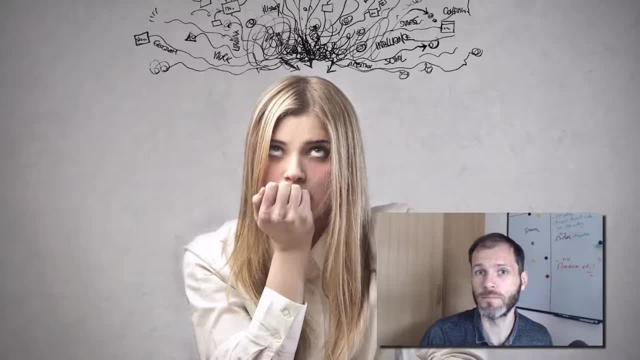 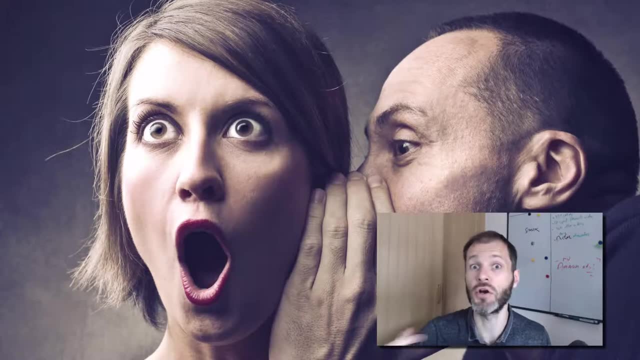 did something in work and something unexpected happened. Another type of writing prompt you can use is to write about something that shocked or surprised you, or something that turned your world upside down. So this could be something somebody said to you, or it could be something unexpected that happened, or a sudden change of fortune, like the time a job didn't work out, or 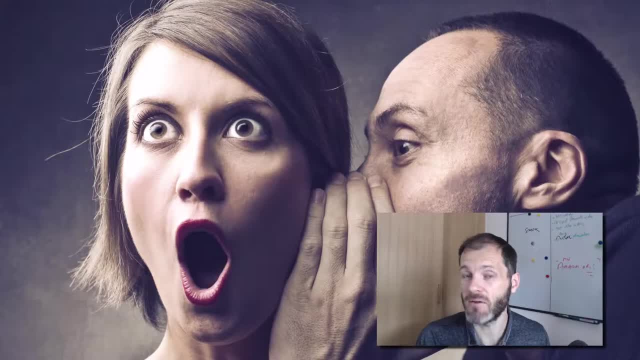 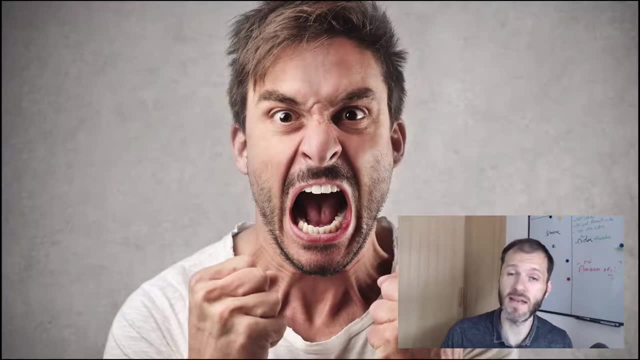 the time you thought one thing about somebody, but then you found out something else about them. Another type of writing prompt that you can use- and this is one that I sometimes like to use, and I know it's one that comedians use- is to write about what makes you feel angry. So if you've 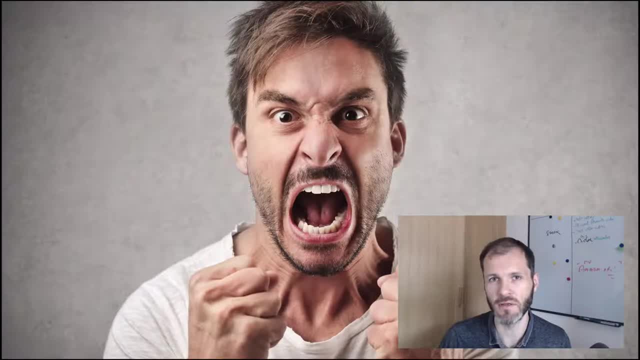 ever sat down in front of a blank page and you've tried to write something and you felt a little bit uninspired, or the entire process has felt a bit grey and bland and boring. think of something that fires you up. It could be a person that you met. it could be 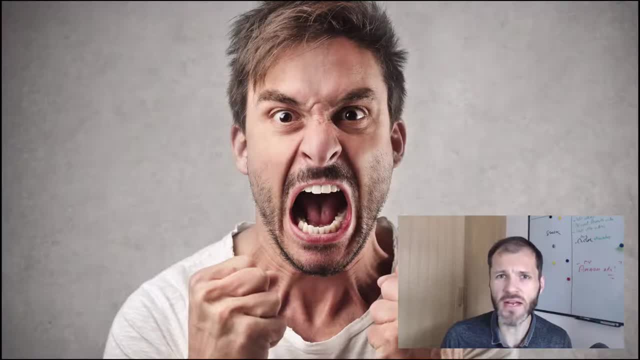 something that happened to you a few days ago. it could be a way of doing things that you really disagree with, or it could be an idea that you're firmly against. So write about that, dig a little bit deeper into that angry emotion and use that to fuel what you put down on the blank page. 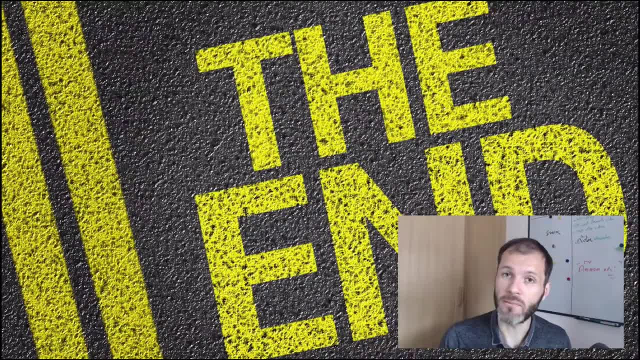 And, of course, another way that you can use a writing prompt is to write about the end. So, rather than starting at the start of your book or your story, write about how you want things to work out. Write the final scene, write the last sentence, because when you write at the very end and work backwards, 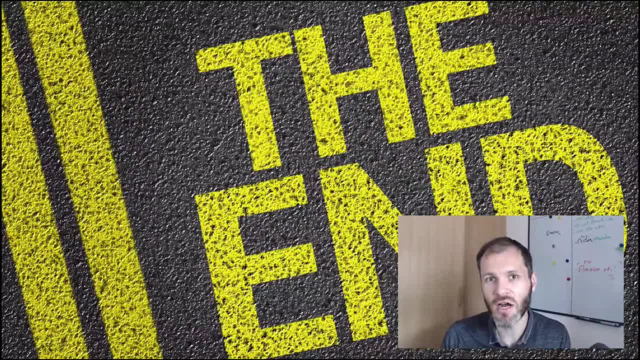 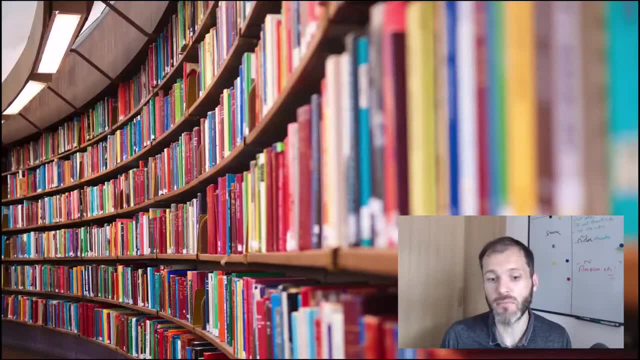 it turns things upside down and it makes it that bit easier to get started and to get going. Of course, these are just some of the types of writing prompts that I like to use, but my biggest tip for you is actually to build your personal library of writing prompts.